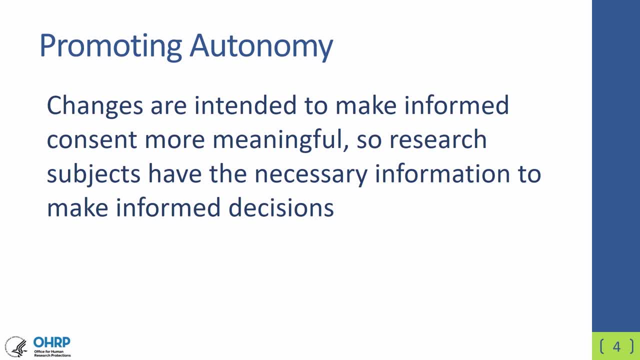 make a decision about what they really want, what best serves their interests, and we want to make sure they have the necessary information conveyed in an appropriate way to allow them to make appropriate decisions based on their own values. So that's the goal and there's a recognition. 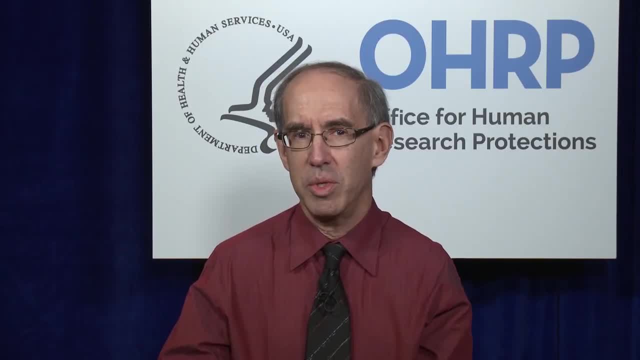 that for decades, people have discovered various reasons why consent forms and consent processes are not doing what they ideally could best do in terms of serving that. Consent forms have been complicated, often have a lot of boilerplate and we could improve things, and that's the purpose of most of these changes. 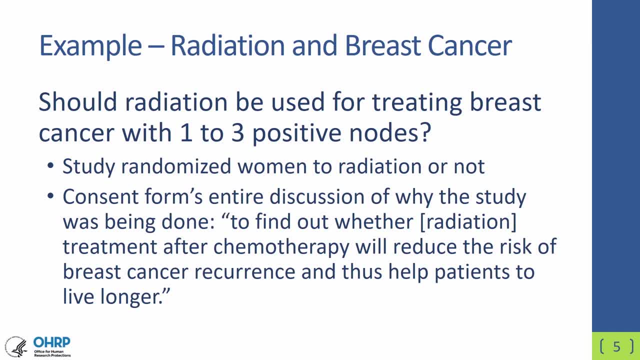 And to explain this, I want to frame it by giving you an example, and hopefully this example will give you a sense of what's going on, sense of what the changes to the new rules are designed to accomplish in terms of remedying some defects, deficits in the current rules. 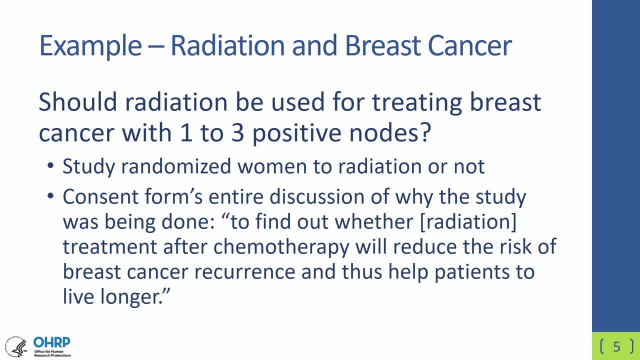 And so the example is actually a real study that took place quite a few years ago, and it was about a research study, a clinical trial, involving women who had breast cancer And, in particular, these women had undergone surgery. They were undergoing chemotherapy And, as a result of the surgery, they knew that the breast cancer had spread outside. 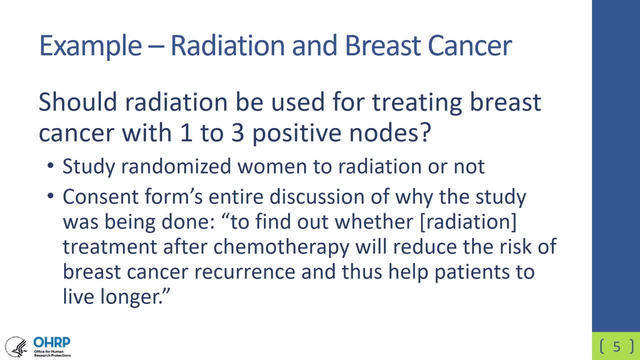 of the breast and they had between one and three nodes that were positive, that demonstrated the cancer had spread to it, And the study was randomized. and the question was: should these women get, in addition to the chemotherapy and in addition to the surgery, radiation, local radiation. 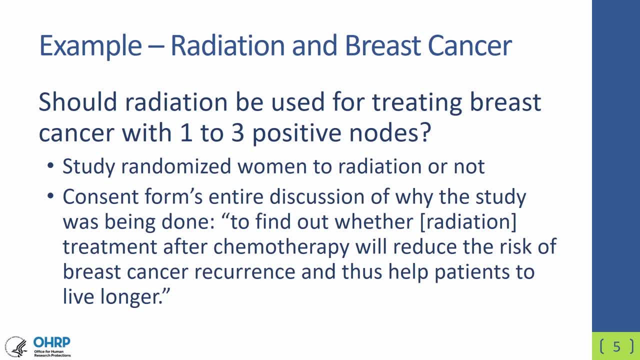 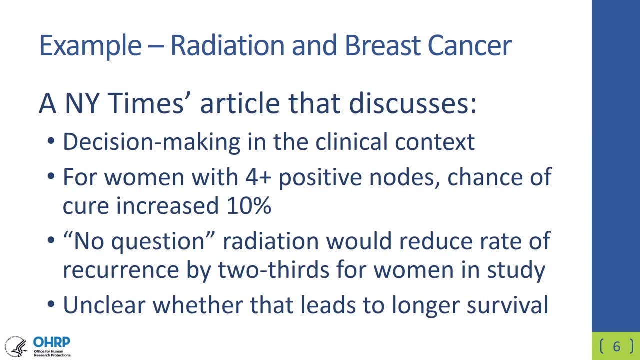 And the consent form had basically one sentence, which was its entire discussion of why the study was being done, and it was to find out whether radiation treatment after chemotherapy will reduce the risk of breast cancer occurrence and thus help patients to live longer. And what's helpful in terms of looking at this study is there was actually an article. 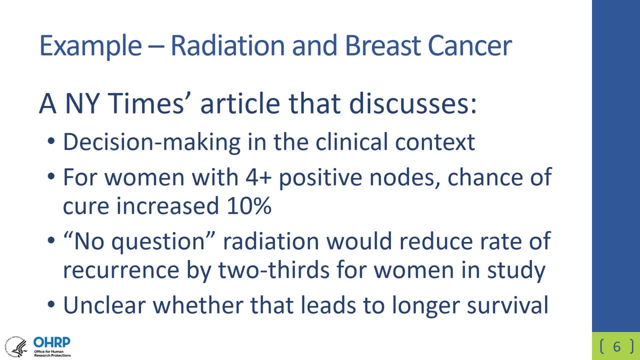 that showed up in the New York Times that was discussing not the study, but what was actually happening in terms of clinical discussions between patients And their physicians about this same scenario. In other words, you were a woman who had between one and three positive nodes, and should you? 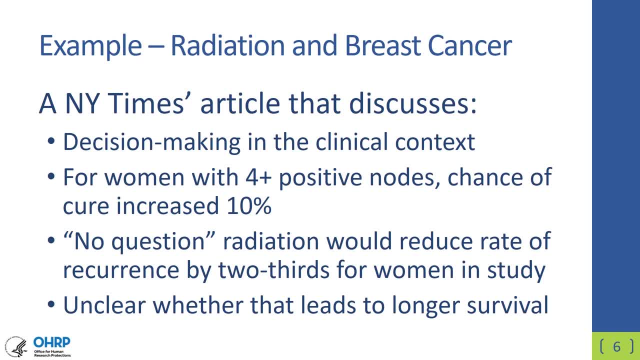 or should you not get radiation? And it wasn't actually a very long article because I want to encourage you to think about the difference between getting consent in a clinical context and getting consent in the research context, And I think one of the major goals of the new rules is particularly for people enrolling 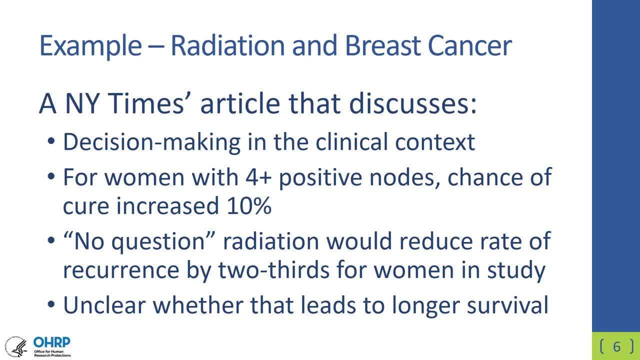 in considering enrolling in clinical trials is to make the decision about whether or not they're going to get radiation, And I think one of the major goals of the new rules is particularly for people considering enrolling in clinical trials- is to make the decision about whether or not they're going to get radiation. 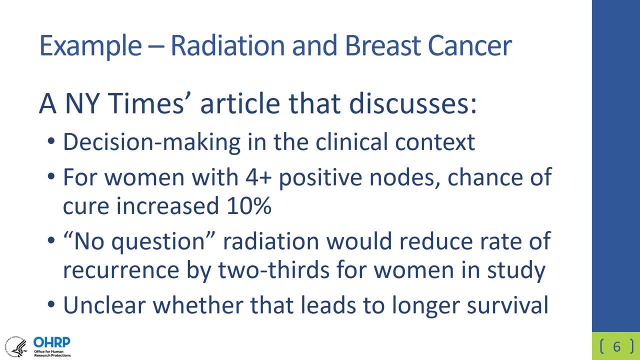 Also, it was much more complicated than your average decision-making about enrolling in a clinical trial, more similar to the way people think about any other type of clinical decision. So, in any event, you had this New York Times article and it again was only about decision-making. 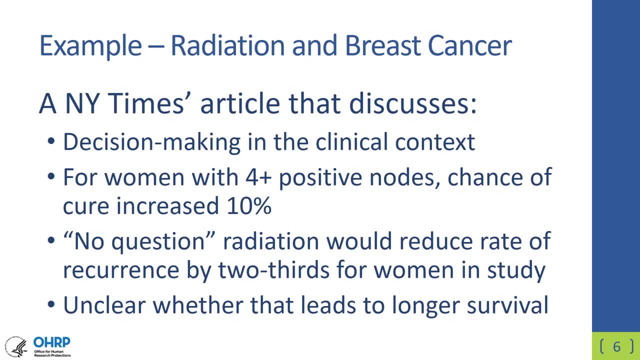 in the clinical context and it actually had a lot of information. It wasn't very long but in spite of that it had a lot more information than you would have received from actually reading the consent form for the research study, And normally we think research actually does a much, much better job than clinical consent. 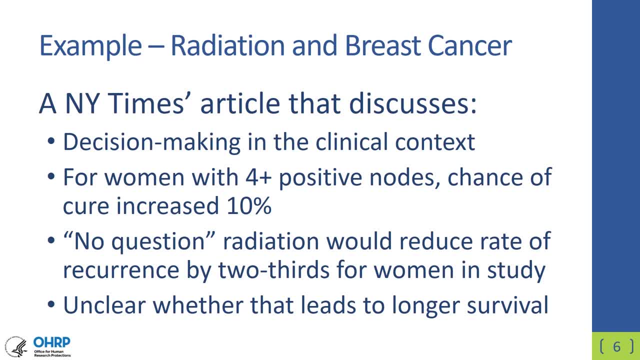 And here you sort of saw the opposite, And it told you a number of things, including that there was no doubt that getting radiation would reduce the rate of recurrence of the cancer returning by 2 thirds for the women in the study. The thing that was unclear was whether or not 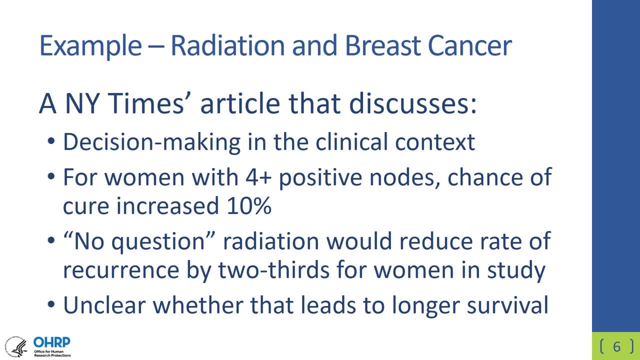 that would actually allow the women to live longer. So that was uncertain. Again, none of this information was really conveyed, at least that the 2 thirds reduction in recurrence was not conveyed in the consent form for the trial. And so this raises the question: should that sort of information 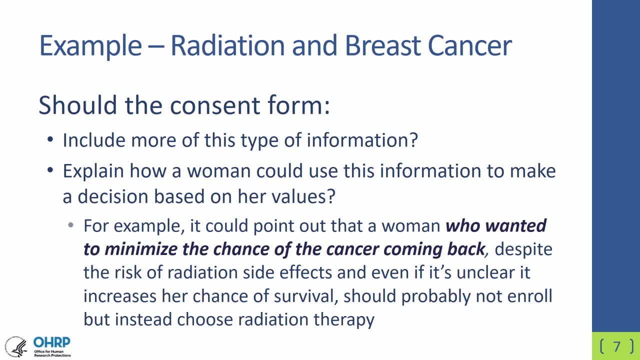 been in the consent form And in general, should we be including more of this type of information? And just to think about it, how might a woman use this information and what might a consent form tell a woman to help her make a better? 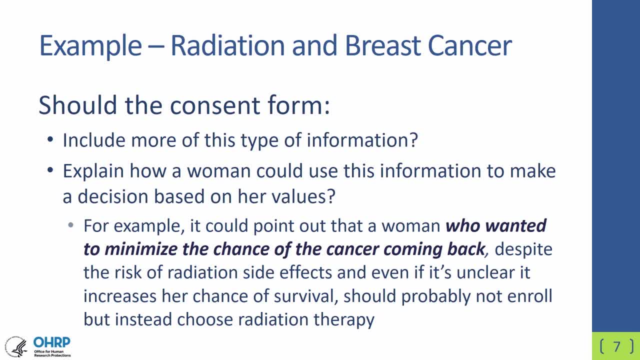 decision. So, for example, a consent form could have pointed out that if you're a woman with a certain set of values, namely you wanted to minimize the chance of the cancer coming back, despite the risk of the radiation side effects, and even if we're just not sure whether minimizing 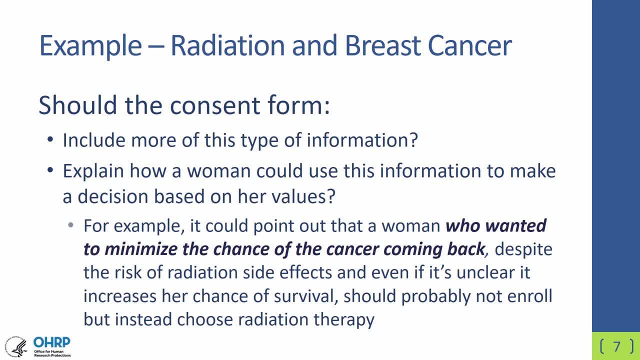 the chance of the cancer coming back will increase her chance of survival. if you're a woman with that sort of value that you just really, really never want to have, a year from now, two years from now, three years from now And you're just going to be in the trial. 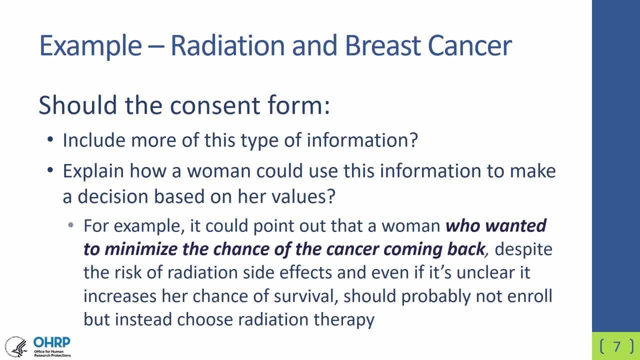 learning that the cancer's come back, then you probably don't want to enroll in the trial, but you probably want to just get the radiation therapy, because we know that the radiation therapy will in fact minimize the chance of the cancer coming back. 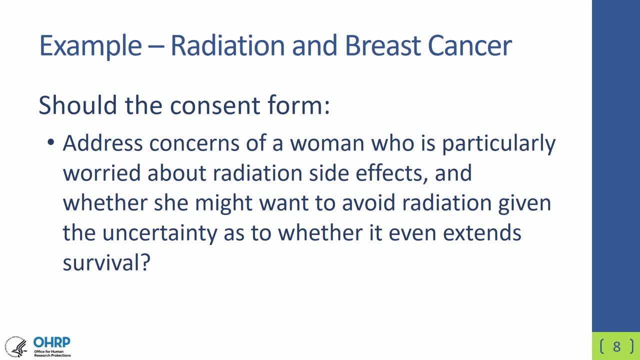 On the other hand, you might be a woman with a different set of values, a woman who particularly is worried about the radiation side effects, the permanent bad consequences to skin underlying tissues. You might be the kind of woman who wants to avoid those side effects as long. 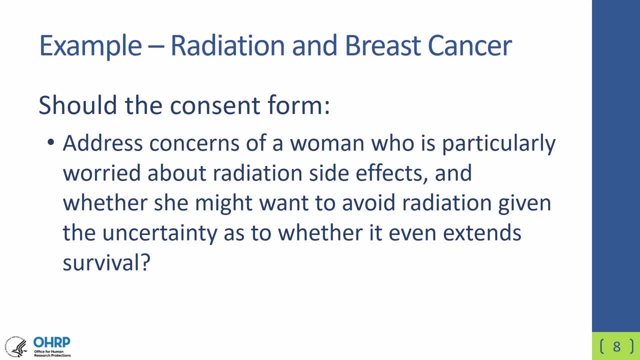 as there is uncertainty as to whether or not getting that radiation will even be good for you in terms of extending your life and allowing you to live longer. So these are sorts of things that the consent form actually could spell out, And then it could go on to discuss. 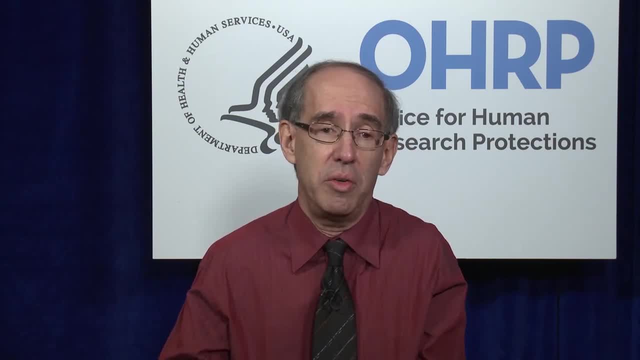 you may be a woman who doesn't have a strong feeling either way and isn't even certain which of these options you want, in which case it would be a perfectly reasonable thing to be in the study, Or you might, in particular, be very interested in helping. 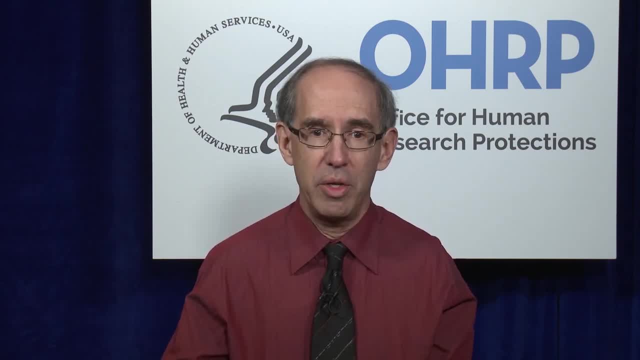 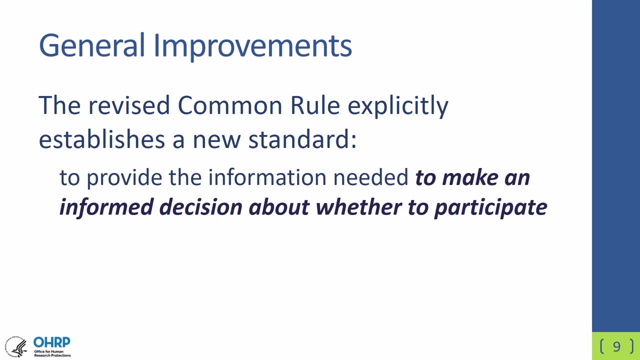 learn more information that will benefit future women- Again, another good reason for being in the study. So that's sort of a background way to think about this. And now let me get into the specific changes in the revised common rule, And one of the new standards is specifically 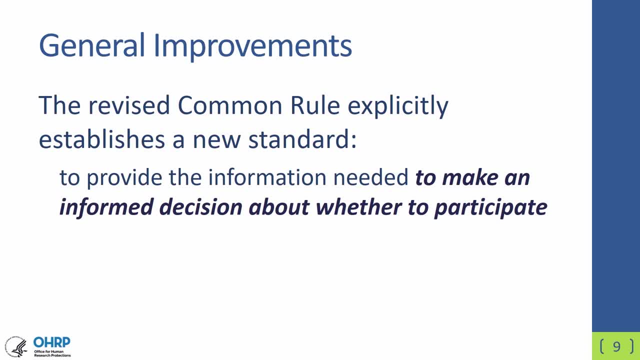 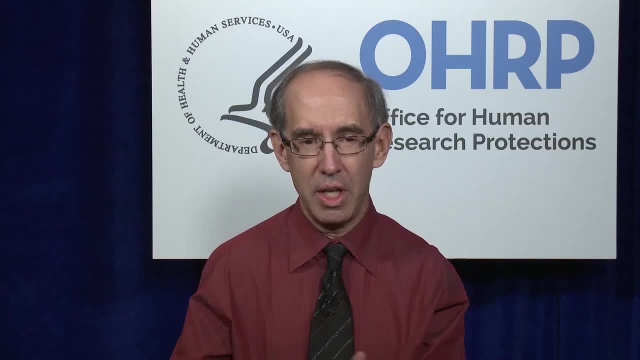 spelling out that a consent form and the consent process should provide the information needed to make an informed decision about whether to participate. And again you'll see the key And a number of the changes is about treating this as a decision- in many ways, similar, certainly. 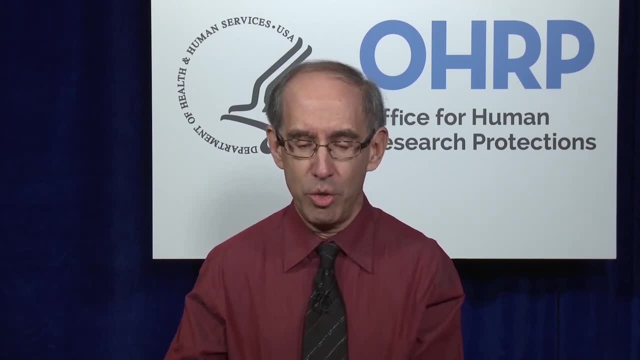 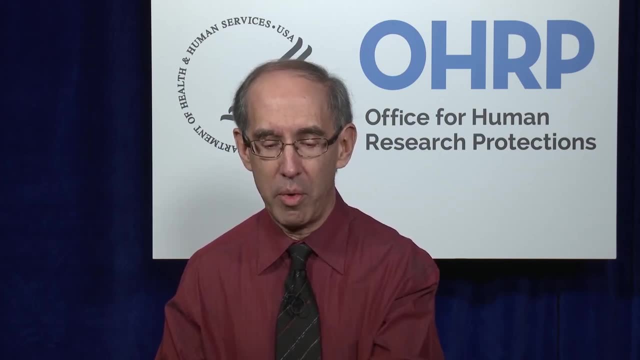 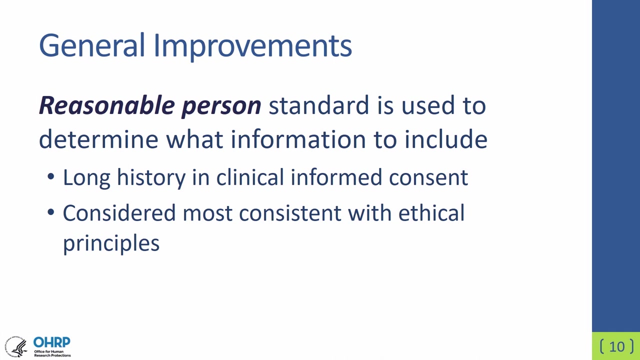 for clinical trials, which I'll concentrate on here- similar to a clinical decision and giving a person the information needed and highlighting their options and what they might want to think about. Another change is introducing the reasonable person standard, And this is going to be used to determine. 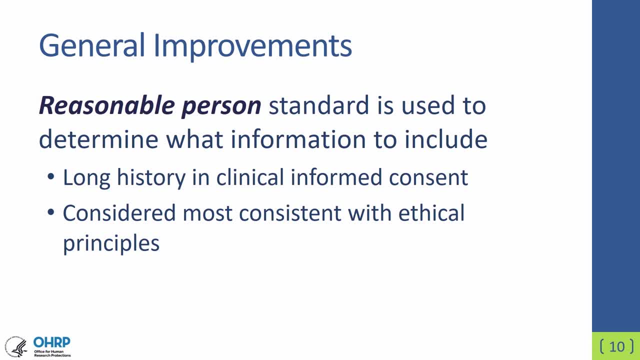 what information to include, And one of the reasons for including this is that this has been used as a standard in the legal context for clinical informed consent And it's considered most consistent with ethical principles. And in particular, just so you understand what this is about, 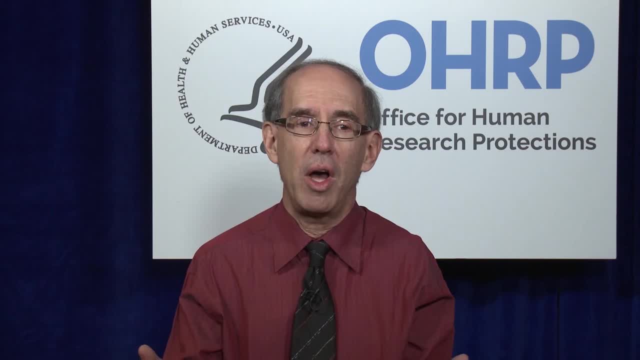 it's not going to resolve every gray line in terms of which piece of information you might want to include, But what it will do is give you a better sense of the really big ticket items, The major pieces of information that certainly could be disclosed. 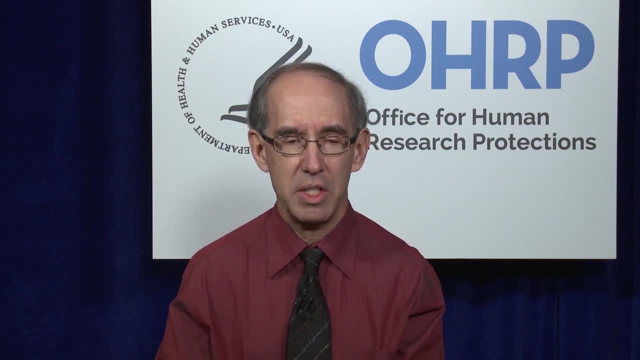 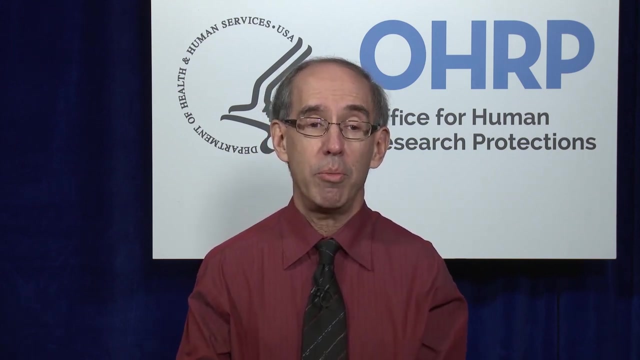 And to understand that the contrasting standard that is actually still used in quite a few states is what's called the professional standard, And what happened under professional standard is: if there's a dispute about whether a particular piece of information should be conveyed, you look to the profession, in this case, clinicians. 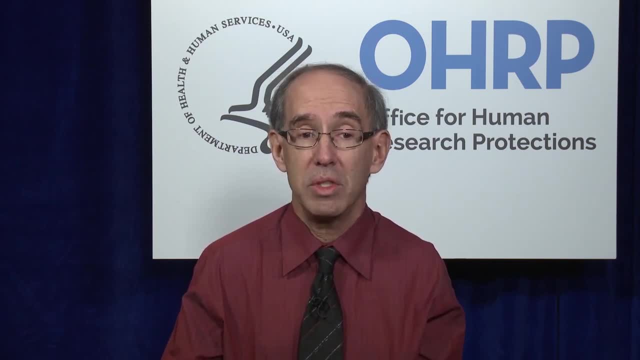 and you ask: what do they generally disclose? And if they didn't disclose a particular piece of information, then you're out And then end of the discussion, Whereas the new reasonable person standard says: let's look at what your average person who's. 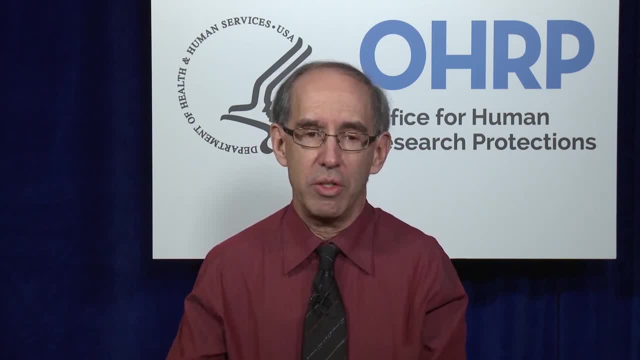 in that scenario, the person with breast cancer- if it's a breast cancer study, would they want to know about this? And to give you one of the famous examples in the legal context, a young man underwent back surgery And it worked out after the surgery. 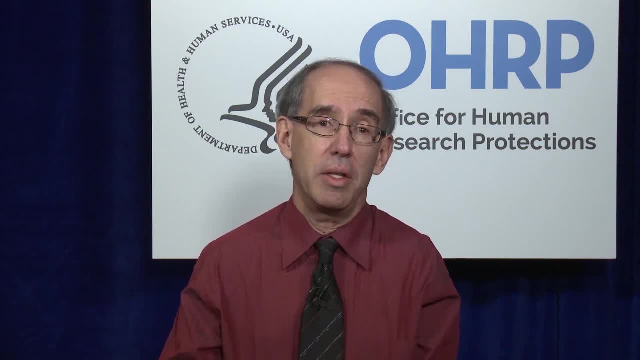 he ended up being paralyzed And it apparently was the case that we knew ahead of the surgery that there was about a 10% chance of being paralyzed And that was not disclosed to him And in fact it worked out that under professional standard, 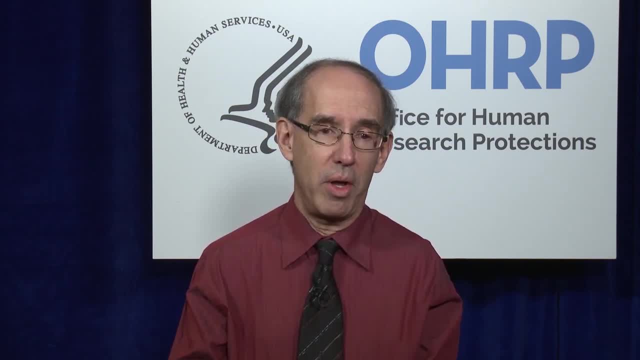 physicians in general weren't disclosing this, And so the bottom line is: under the reasonable person standard, it's well, would a person undergoing this surgery want to know this pretty serious consequence And most of us would say, of course. So again, it's not going to eliminate gray lines. 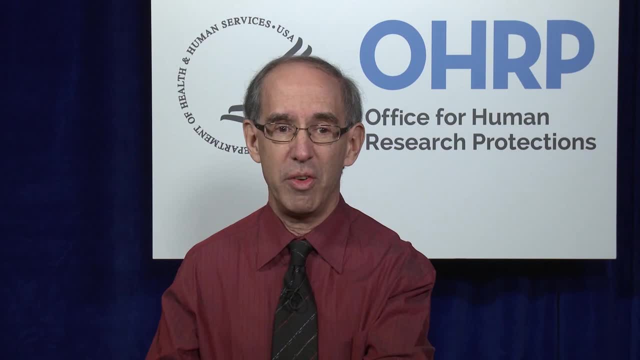 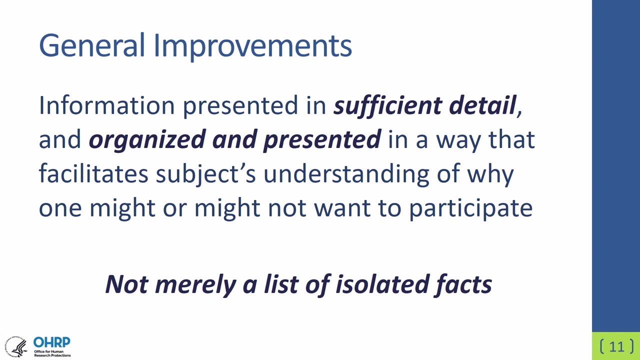 But it will help disclose important pieces of information. Some other changes, Some changes here. The information has to be presented in sufficient detail and organized and presented in a way that facilitate the subject's understanding of why they might or might not want to participate. 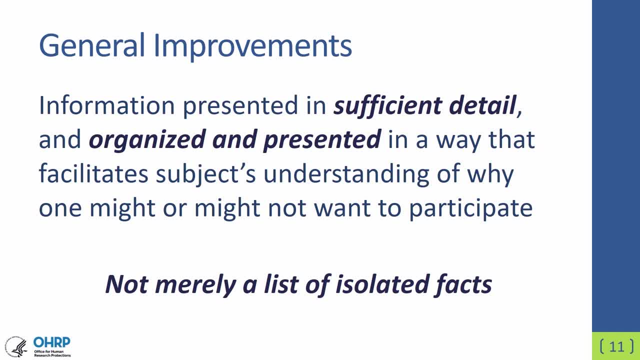 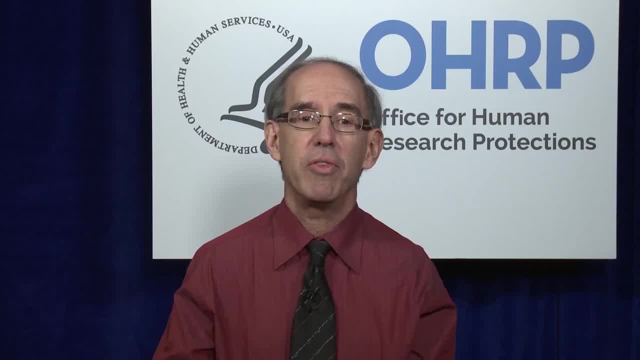 Sufficient detail. It's not uncommon that consent forms- and there have been complaints about this for decades- are too vague. For example, on the benefit section of a consent form, it often can say you may or may not benefit from participating in this study. 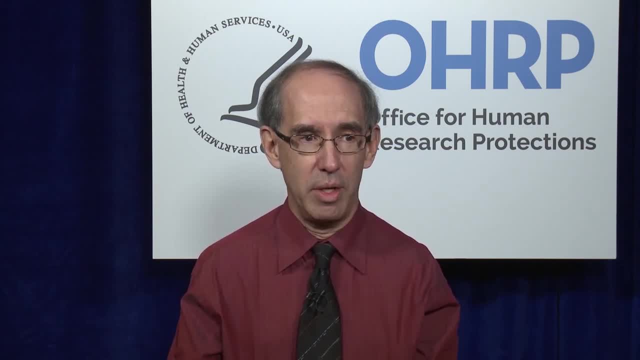 Notice what that sort of language does. It doesn't give you, the prospective subject, a tip off of exactly how likely you are to benefit And many people hearing you may or may not benefit may think it's a 50-50 chance when in a particular study. 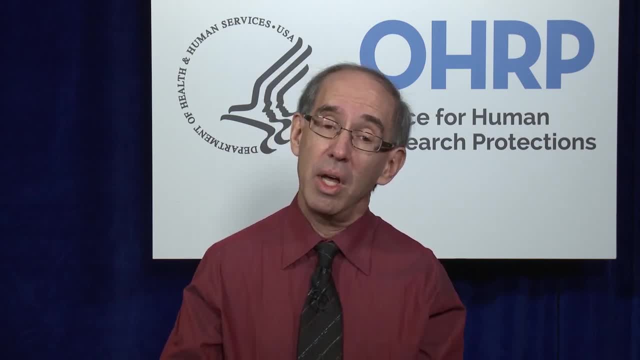 we may know that your chance of benefiting is less than 10%. It also that kind of language doesn't tell you the possibility of a benefit Again in the cancer trial. it's possible that the benefit that's most likely is it. 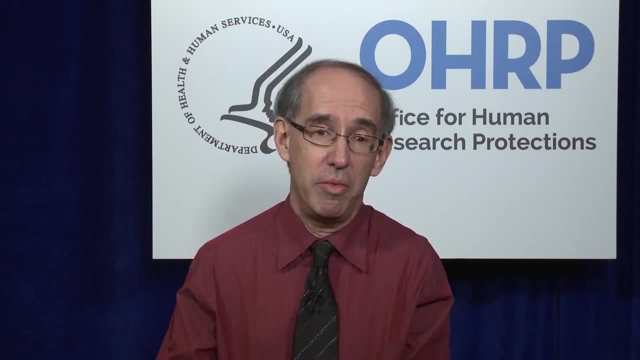 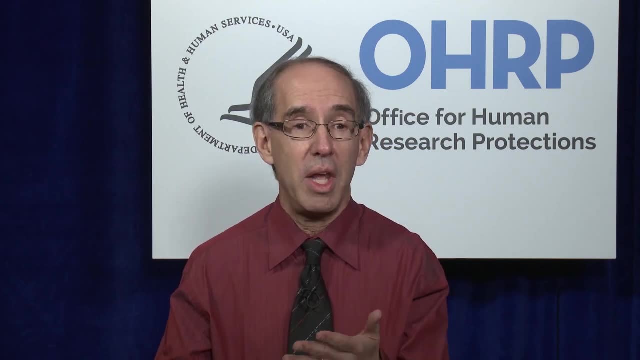 will improve your symptoms, reduce your pain. it may be very, very clear that it's not going to increase your life expectancy, let alone cure your cancer. Yet if you don't tell that to the person, then they have no way of knowing. 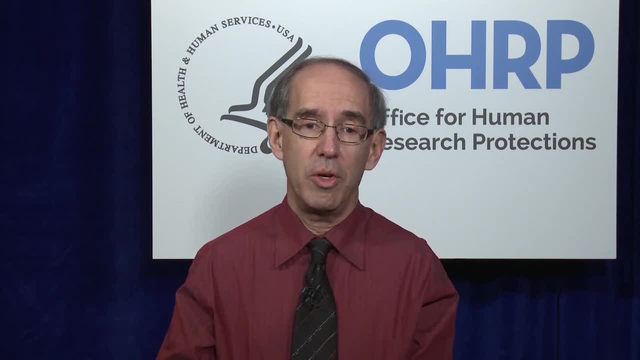 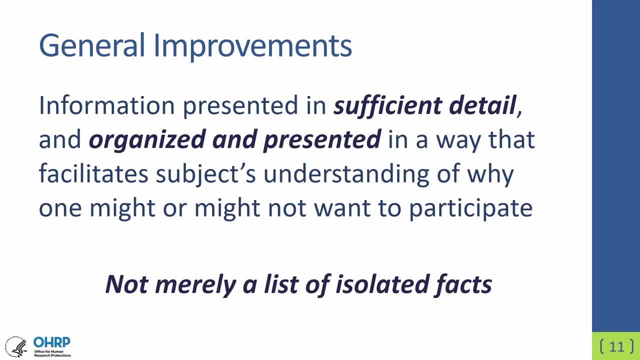 And they may in fact be guessing. well, of course there's a good chance this will cure my cancer. Bottom point on this slide: it should not merely be a list of isolated facts And get back to the discussion of that example. 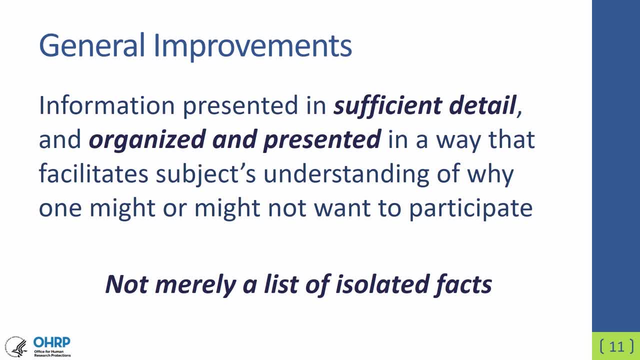 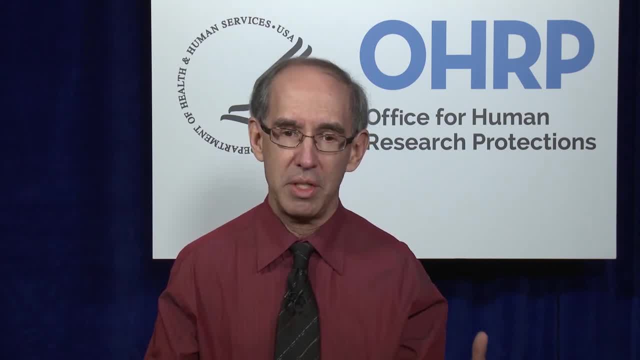 I was giving you Consent forms right now actually are not as good as they could be in terms of being aids in decision making. So having a separate paragraph that's risks, that's benefits, that's alternatives, instead of just those lists of those sort. 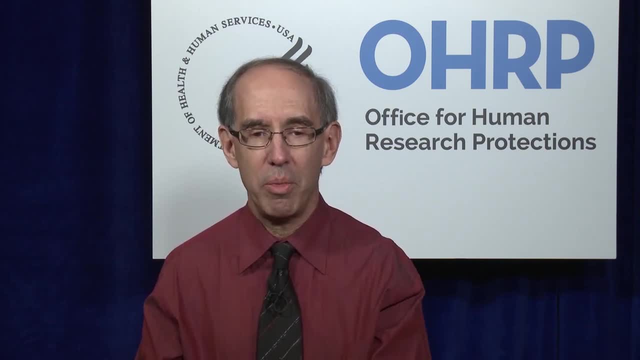 of blurbs, put it all together and try to explain to the person how they should think about this, which often is fairly complicated. The goal is to make it easier for people to make good decisions and help them process this complicated information they're being given. 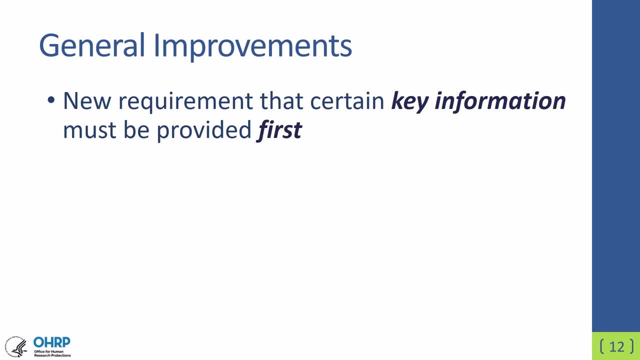 There's a new requirement that certain key information must be provided first And again. getting back to the overview of this, consent forms are very long. They could often be 25 or 30 pages. A person looks at this and their eyes glaze over trying. 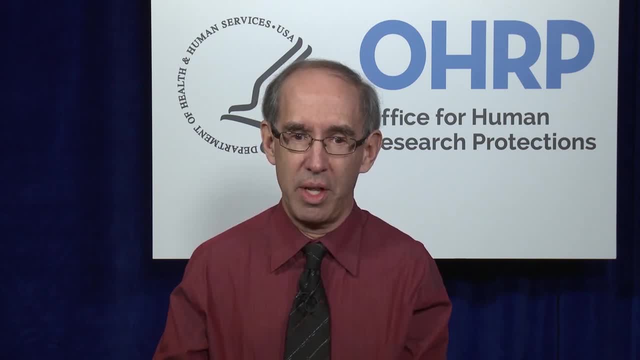 to figure out? do I have even the time to understand this complicated document? And so the sense now is: let's put the really important information right up front in the first two or three pages, Even if people don't read the rest of the form. 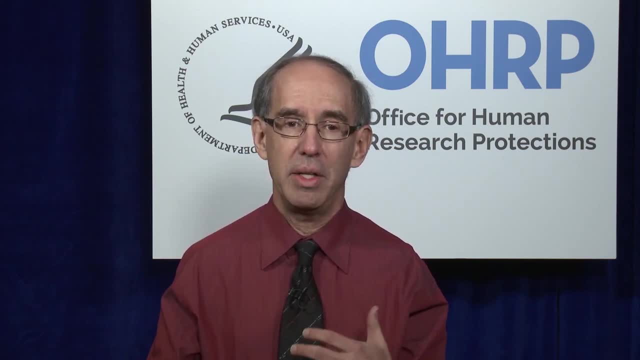 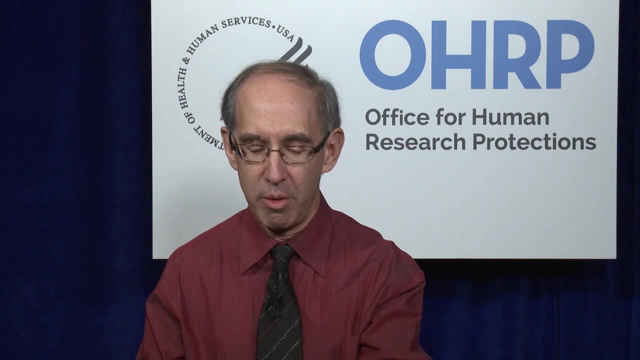 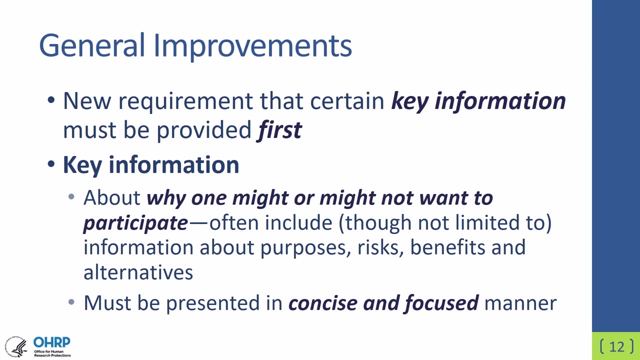 they'll actually have what's important right at the beginning, And it will both include that information and, as I indicated, put it all together, explain to the person how to think about it in terms of reaching a decision. Again, it's about why you might or might not. 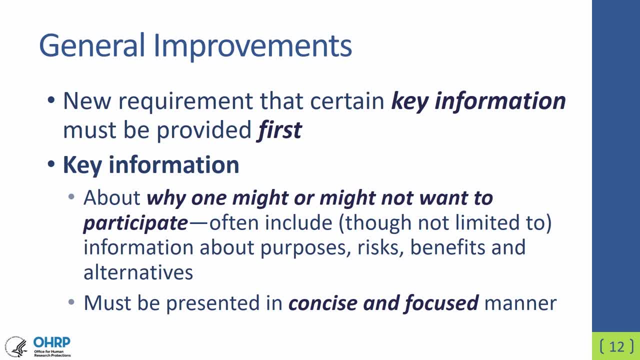 want to participate And often, again, it will include information about the purpose, the risks, the benefits and alternatives And it will put it all together and explain to the person how to think about it. Again, it's about these pieces of information. 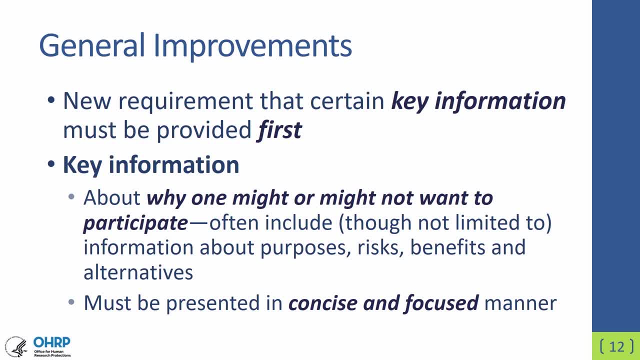 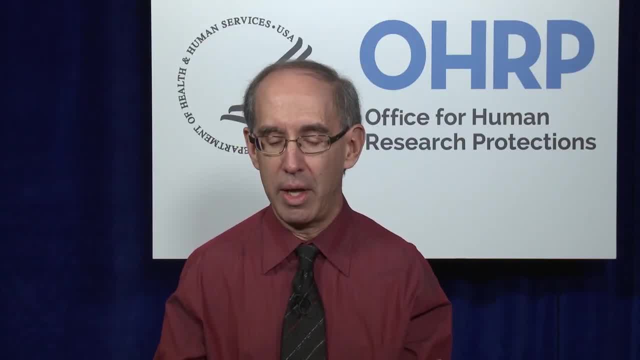 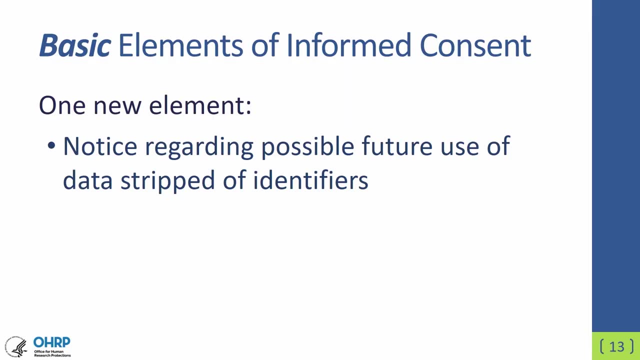 in terms of making a decision, It should be presented in a concise and focused manner. Again, the goal is a few pages at the very beginning of the consent form that a person, hopefully, will look at and will actually read. Now we've sort of covered the general changes. 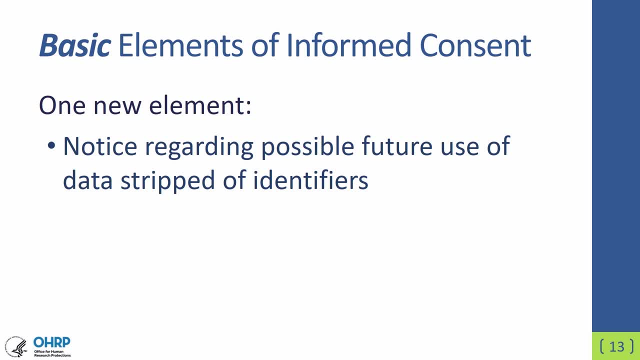 And now let me go on to a few more specific changes And in particular, the changes have been made to the basic and the additional elements of informed consent. I do want to mention that the sections in which you find these lists have been changed. 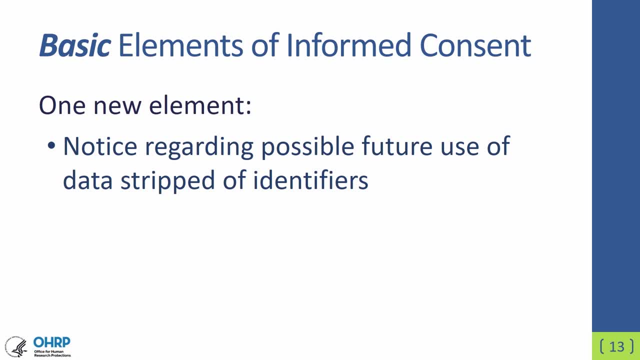 So section 116B is the basic elements of informed consent And section 116C is the additional elements of informed consent. As to the basic elements, there's one new element And that's basically a notice. It's almost less. It's a notice saying that there may be possible future use. 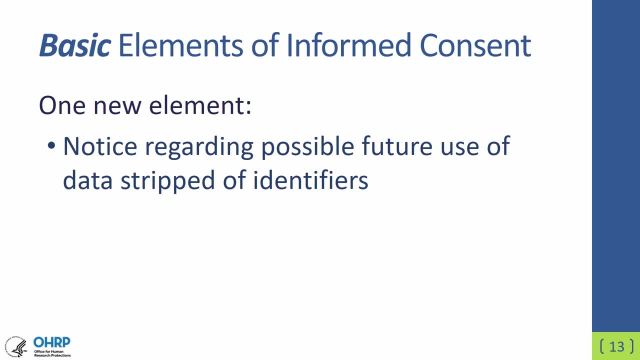 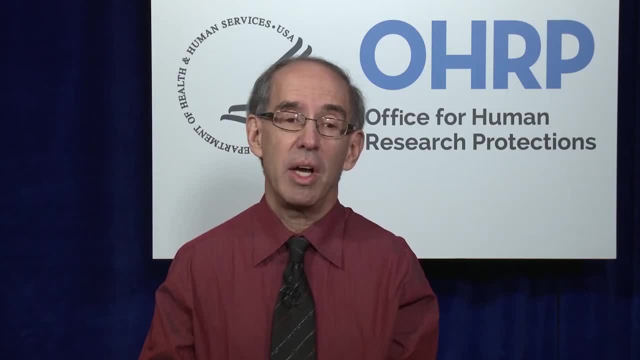 of data, stripped of identifiers, And this is basically increasing transparency and letting somebody know this probably is going to happen And if you don't like it, I mean, your one option is to not participate in this study- But basically, most consent forms. 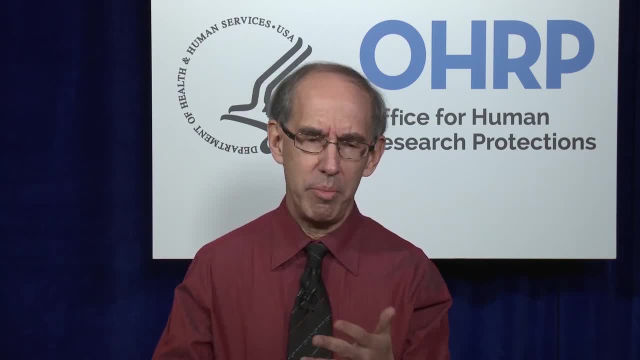 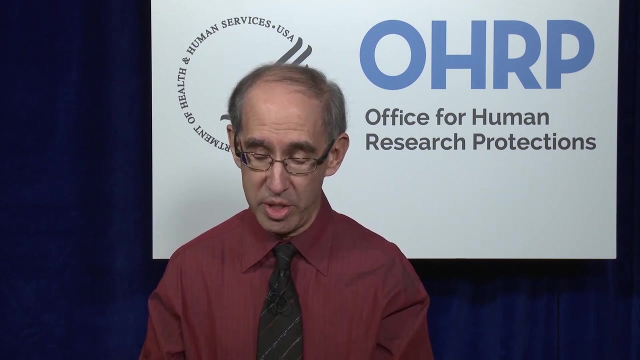 will have to say this or actually otherwise say that they're not going to participate in this study. So that's one thing. The other thing is to make a promise that this will not happen, And probably that's less likely to happen because that's sort of hard to do and somewhat burdensome. 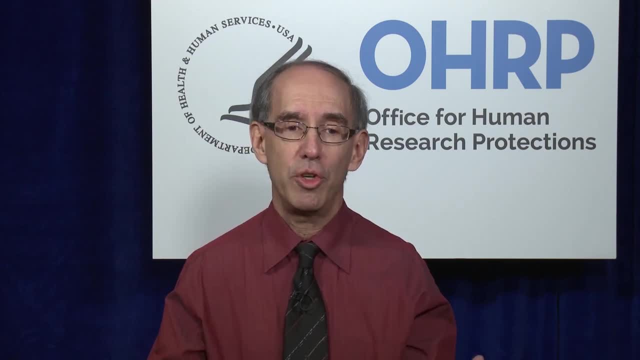 in terms of the research, If notice we're only talking about future use of data stripped of identifiers. If we're talking about future use of identifiable data for future unspecified research, that will generally be covered under the topic called broad consent And there are special rules related to that. 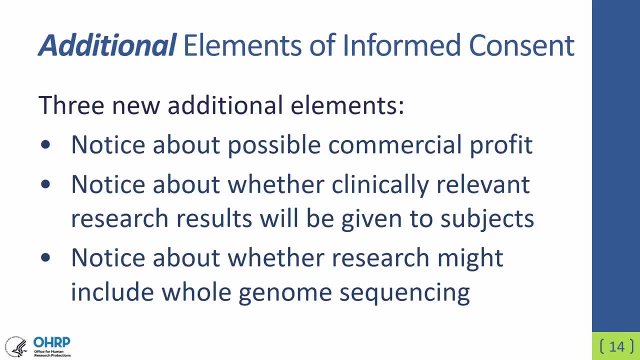 which will actually be discussed in other webinars. OK, so now let me get on to additional elements of informed consent, And here there are three new additional elements. And notice: these are additional elements in many types of studies. You wouldn't actually have to say anything. 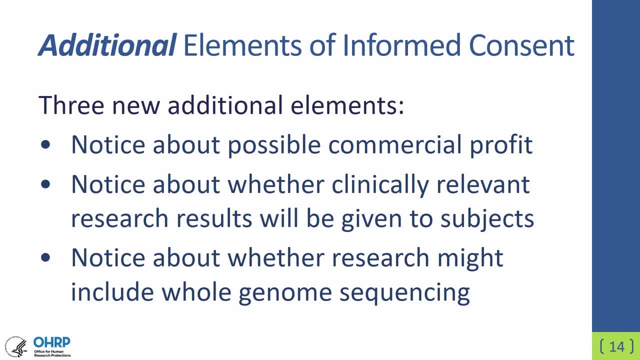 about this if they're just not relevant to the type of study. So you have to give a notice about possible commercial profit again if it's relevant to the study and notice about whether or not you're clinically relevant. research results will be given to the subjects and a notice about whether research 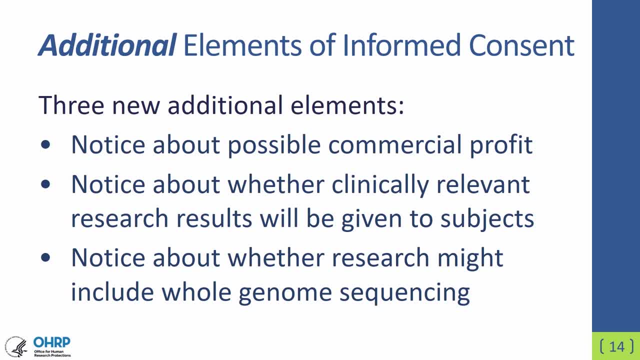 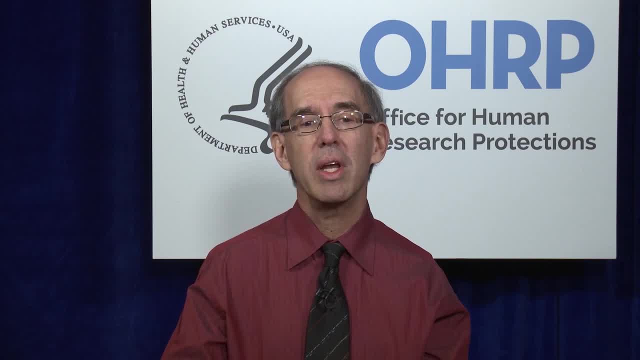 might include whole genome sequencing. Let me say a little more about returning of clinically relevant research results. The goal here is that a subject shouldn't be enrolling in a study thinking they're going to get certain piece of information from the study relevant to their clinical health. 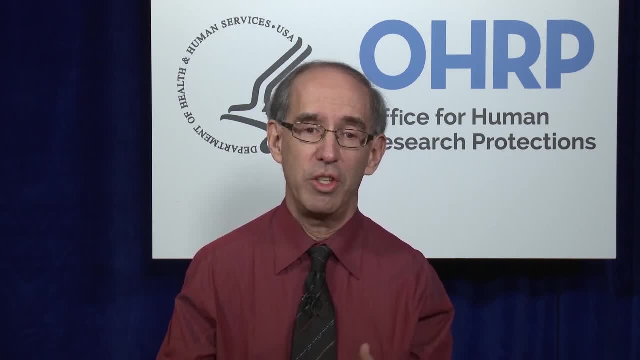 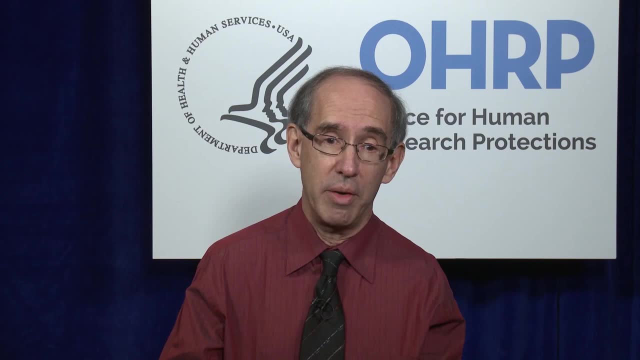 clinical care if that's not going to happen, And so basically you should be disclosing if that won't happen. So, for example, a study might involve doing whole genome sequencing And of course then it would have to tell you that will happen. 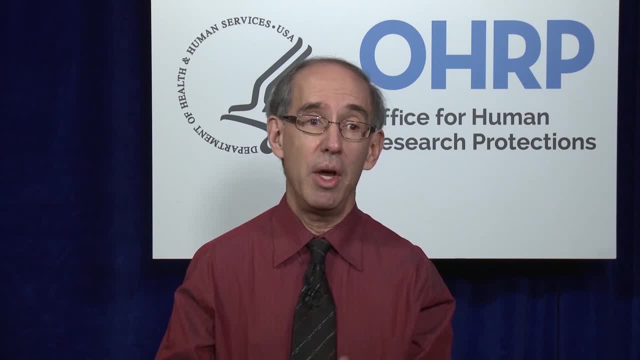 But if it didn't say anything about return of results, a person might think, wow, in this study I'm going to have my whole genome sequenced. That would cost me thousands of dollars to do on my own. I'm going to look forward to getting the results. 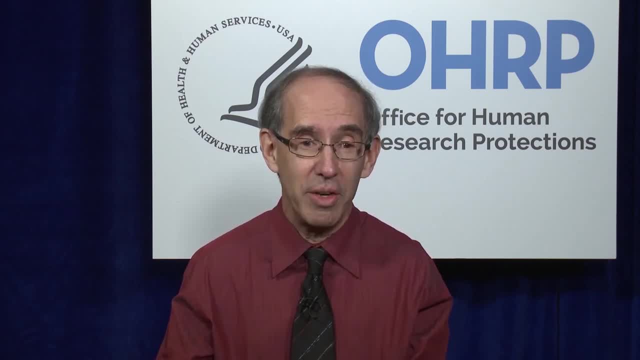 Well, it could be that the study isn't going to let you. It's going to do that, but they're not going to tell you the results of the sequencing. So the new rule says: basically, you would have to disclose that, that you weren't. 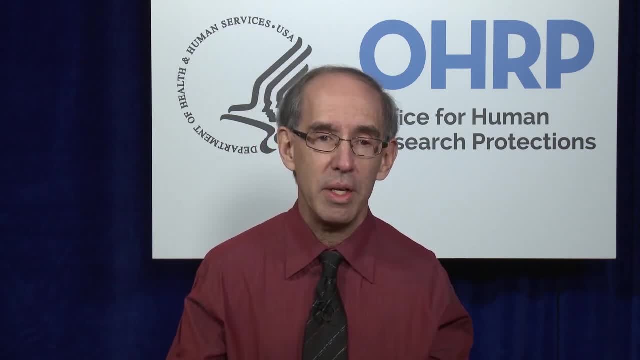 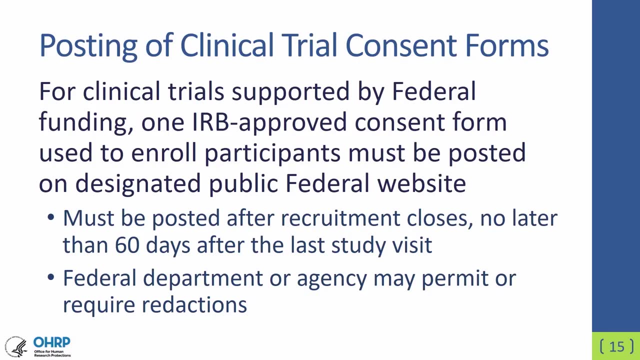 going to return those results. So that's it in terms of the additional elements. Let me go on to another new change, which is- and this is something brand new- posting of clinical trial consent forms. So we're only talking about consent forms. 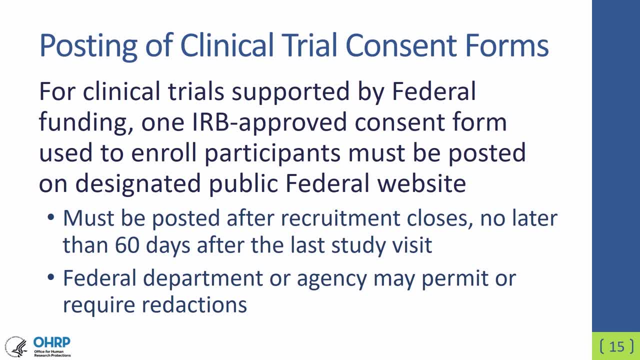 from clinical trials And for a clinical trial supported by federal funding, one version, one IRB-approved version of a consent form that's been used to enroll participants must be posted on a designated public federal website for posting of consent forms, And there's a particular time period during which it. 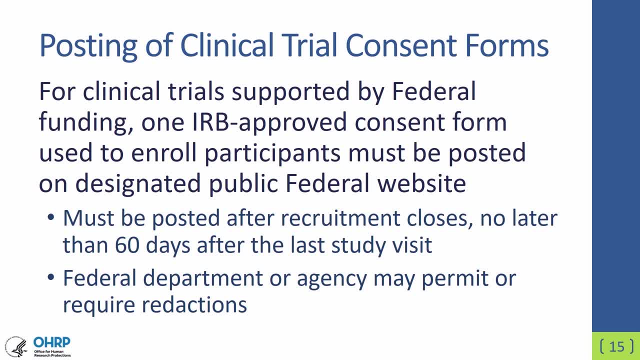 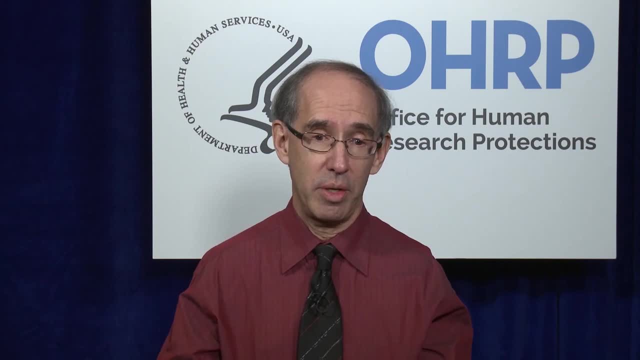 must be posted. It has to be posted after recruitment closes and no later than 60 days after the last study visit. Federal departments or agencies may permit or require redactions And certainly it's open to the people conducting a research study to ask the particular. 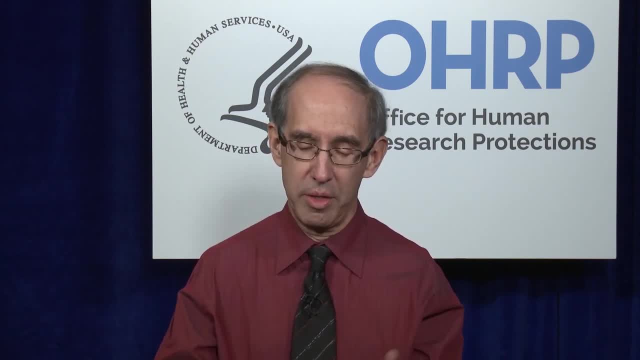 DR. Thank you, MR funding agency and say: could we redact certain types of information Notice based on the posting period? it's after recruitment closes. So the purpose of this rule is to make it more transparent about what types of consent forms are being used. 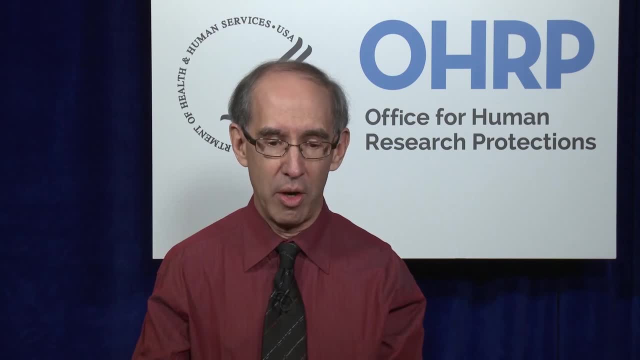 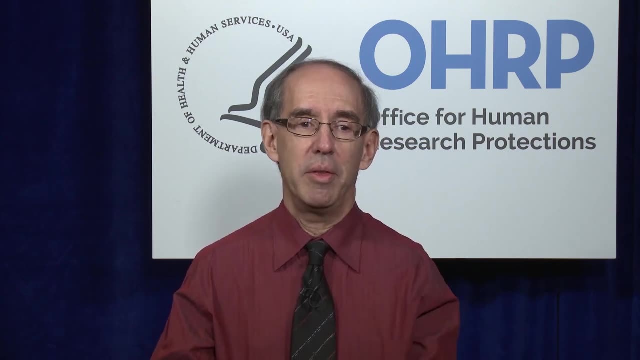 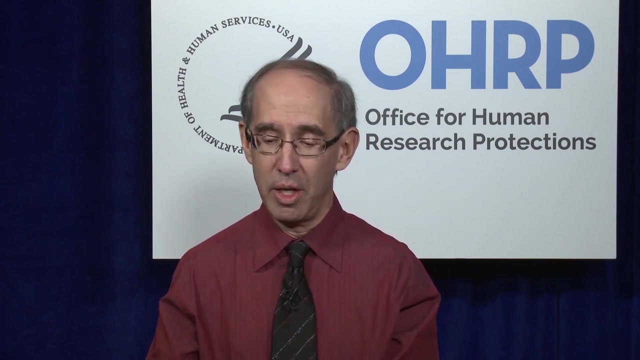 and, over time, improving those consent forms as people see what they are and see good examples. It's not designed to benefit a specific person in terms of while they're thinking about being in the study, DR, You're right. they wouldn't be going to this, this posting site, to look at it, because they 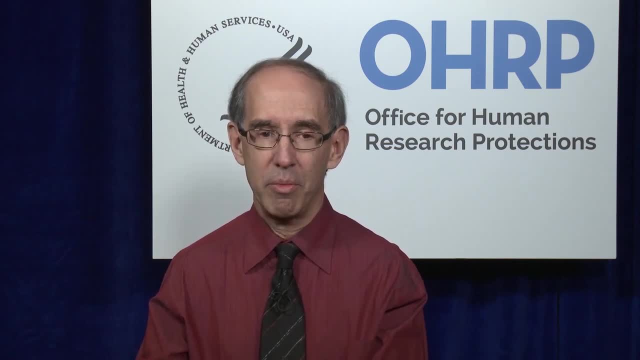 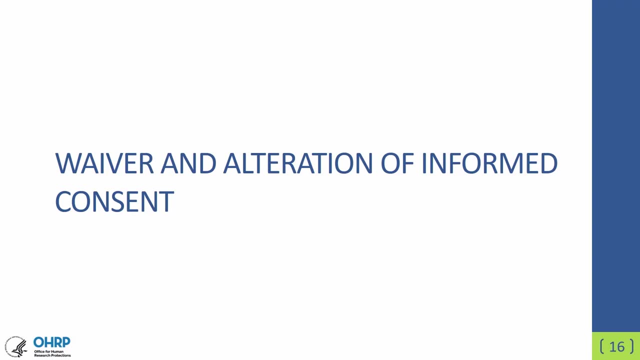 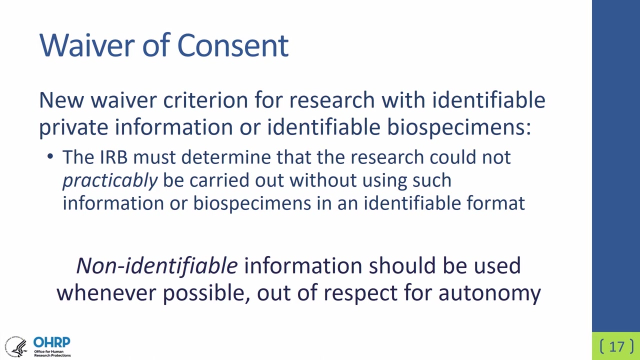 wouldn't find it there because it couldn't have been posted yet to comply with this rule. so that's the posting requirement. now there's been a change in the waiver and alteration of informed consent and, in particular, one new waiver criterion, and this is just for research with identifiable private information or 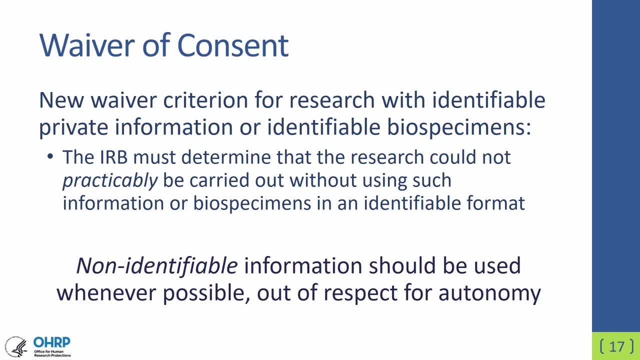 identifiable biospecimens, and in particular, this new criterion is that the IRB must determine that the research could not practically be carried out without using such information or biospecimens in an identifiable format. so the goal here is that, if indeed the research could have been done using 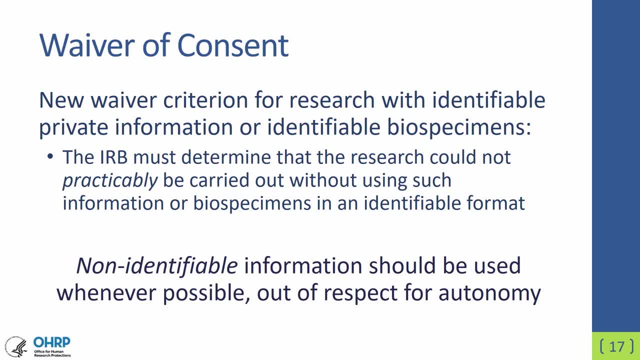 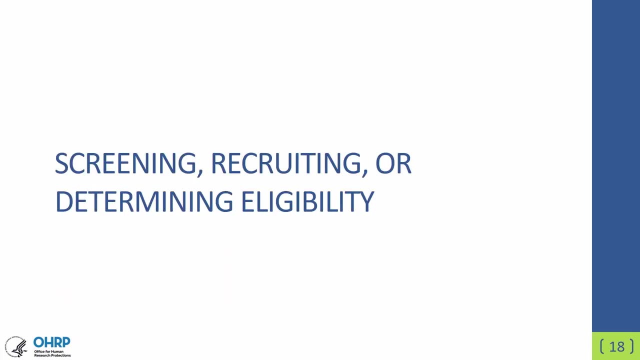 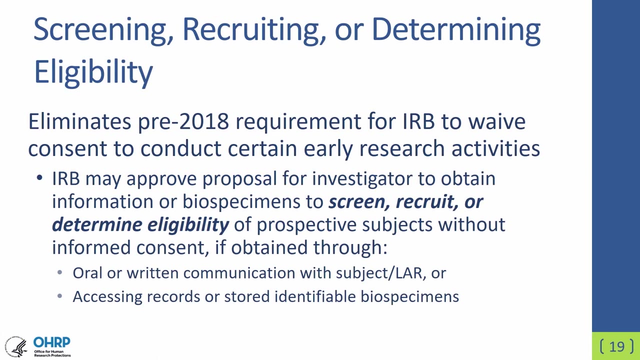 non-identifiable information, then that is in fact what should be taking place, and you shouldn't be then allowing the researcher to use identifiable information, which increases the risk of the research being carried out, and so there's a change in the. the IRB must determine that the research could not practically be carried out. 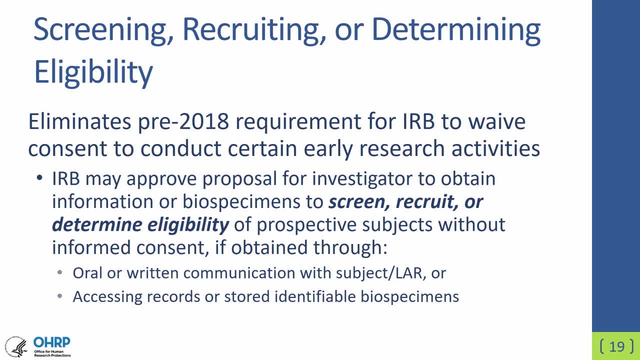 and so there's a change relating to screening, recruiting or determining eligibility and, in particular, what this change is about is eliminating what some people might call a gotcha. that was happening under the old rules that an IRB approved a study that involved certain early research activities. 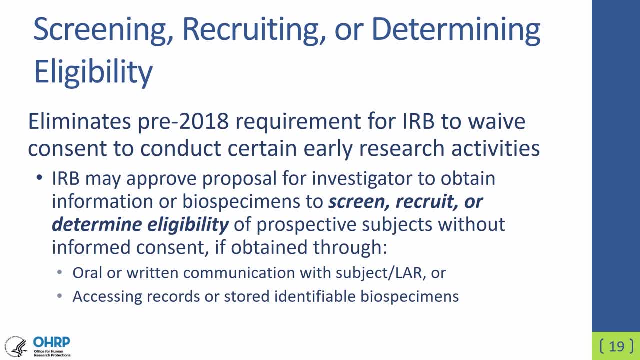 and never specifically waived consent when information is being collected at a point when consent had not yet been taking place, at least meeting all the consent criteria. so under a revision to this, an IRB may approve a proposal for the investigator obtain information or biospecimens to screen, recruit or 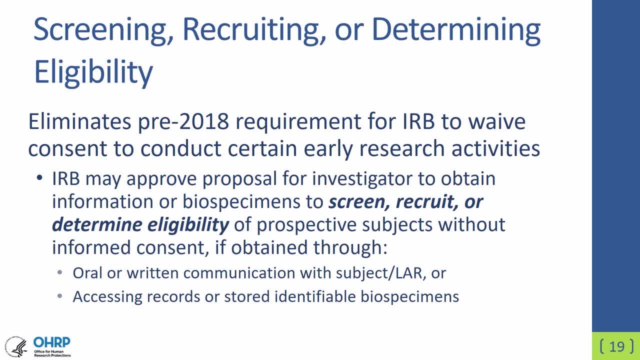 determine eligibility of prospective subjects without doing everything that's required, only informed consent roles if this information is obtained through the two bulleted items here: either oral or written communication with the subject or their legally authorized representative, or by accessing records or stored identifiable biospecimens. 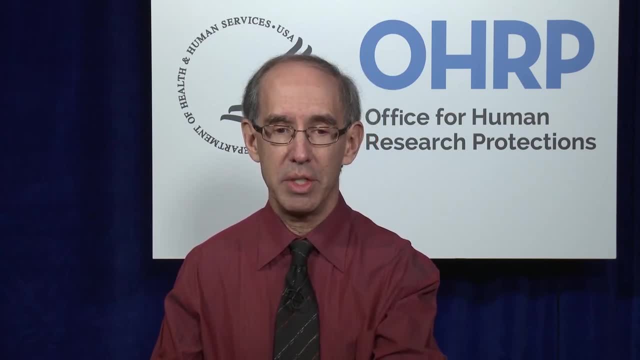 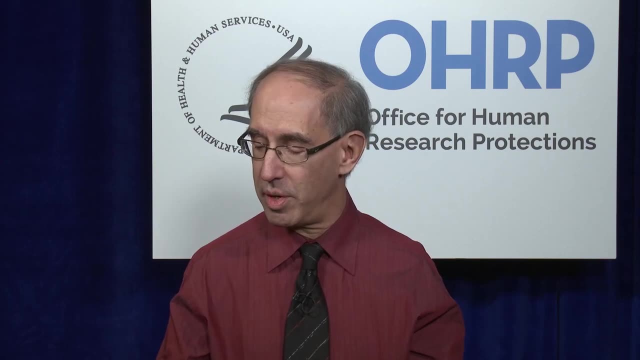 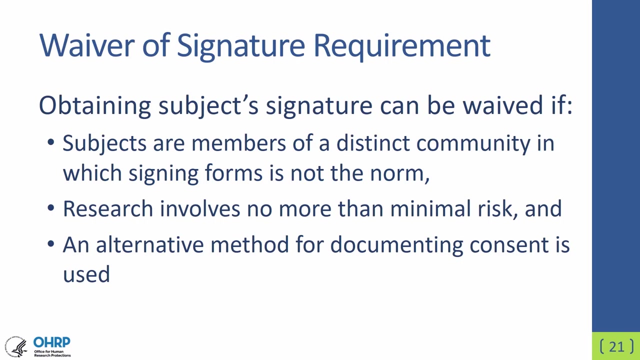 This change actually harmonizes with the FDA rules, which don't require an IRB to be going through a waiver during this scenario. Now there's a change relating to documentation of consent, namely getting somebody's signature before they could be in a study. 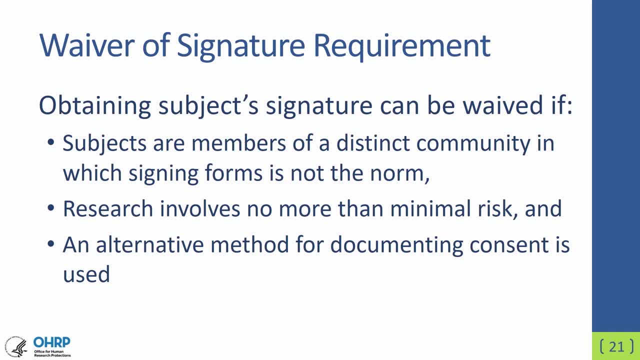 And, in particular, it's an expansion of the waiver of the signature requirement, The need to obtain a subject signature can be waived if the subjects are members of a distinct community in which signing forms is not the norm. the research involves no more than minimal risk and an alternative. 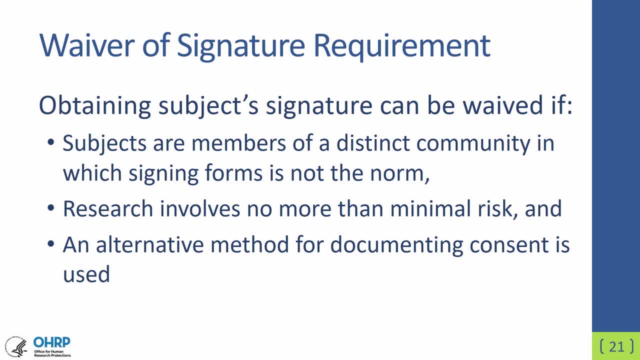 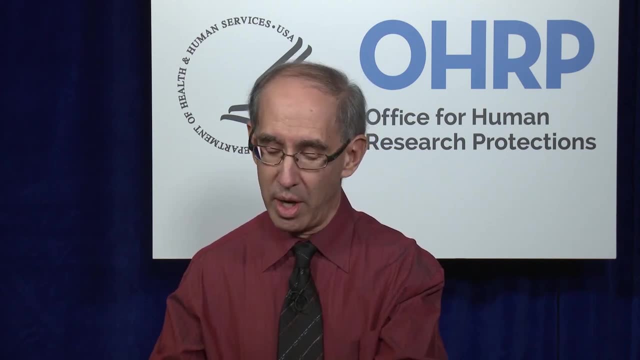 method for documented consent, namely having a record somewhere that this person actually agreed to be in the study and that you know they're in the study. Note that there are other rules relating. you know existing rules relating to when you could waive the signature requirement. 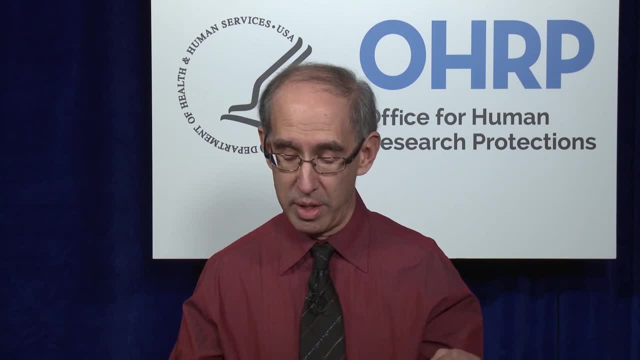 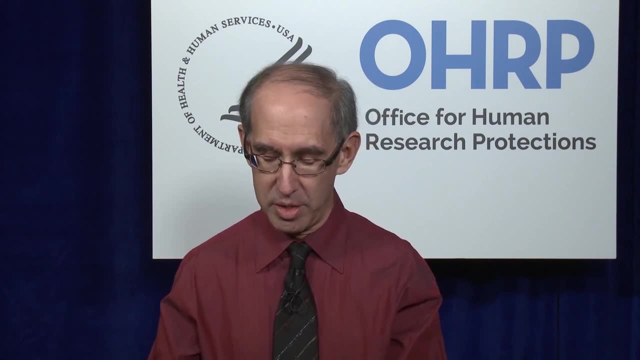 and those still exist. Also note that this waiver can be applied to the broad consent provisions which, again, I'm not going to say much about during this talk, But Likely it would be very rare that it would meet these criteria. Also, the regulations were clarified. 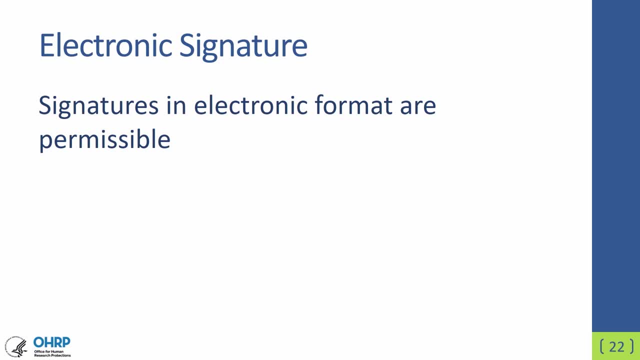 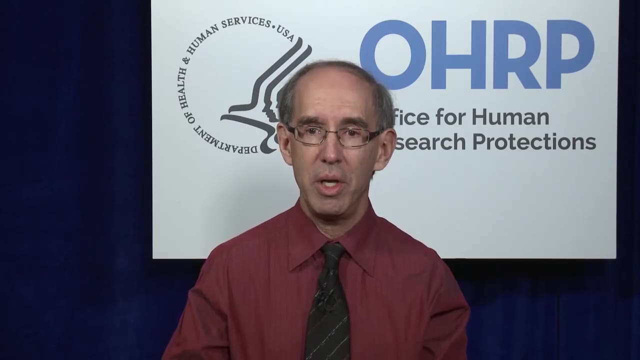 to indicate that it is possible to get somebody's signature in electronic form. That's perfectly permissible. That meets the requirement to have documentation. you know that somebody agreed to be in a study And this is basically just clarifying what people understood the current rules to be. 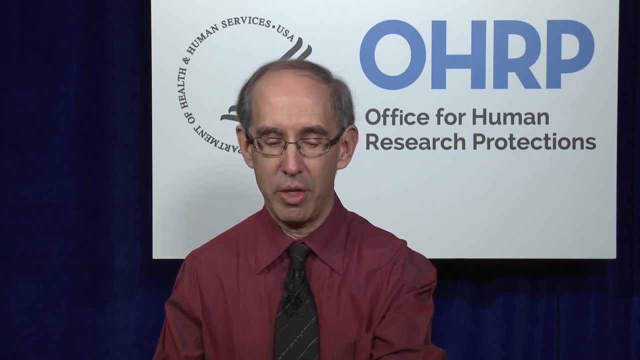 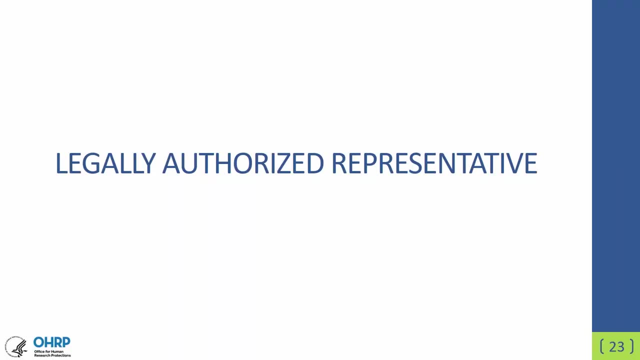 but we just wanted it actually in the regulations so everybody could be Clear about it and there's no confusion about it. So let me now talk about a change relating to when you could have somebody enroll in a study through the consent of their legally authorized 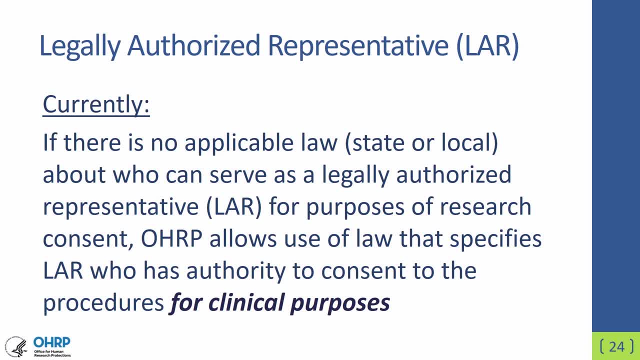 representative, And this is a bit complicated, so let me explain what the current rules are that led to this change. These are the rules under pre-2018 Common Rule. So if there is no applicable law, state or law, local about who can serve as a legally authorized, 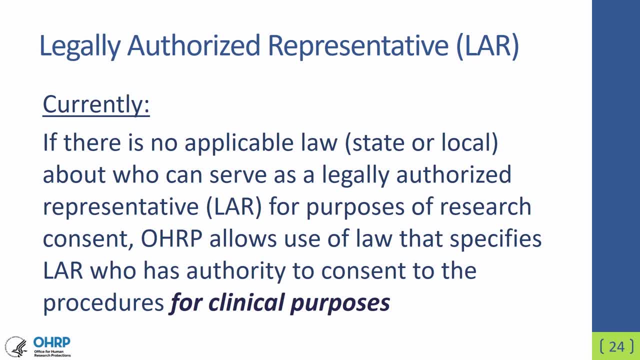 representative, often what's referred to as an LAR- for purposes of research consent. it's the case that OHRP allows the use of a law that specifies a representative who has the authority to consent to the procedure for- and these are procedures that 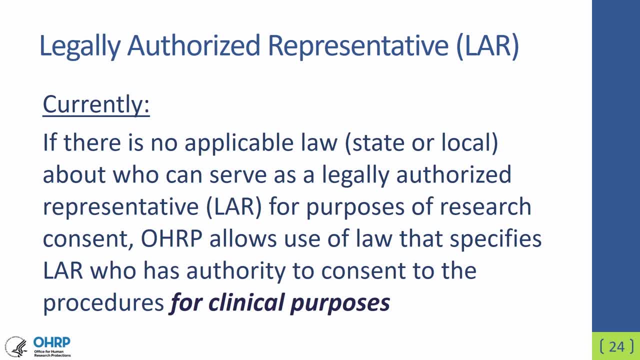 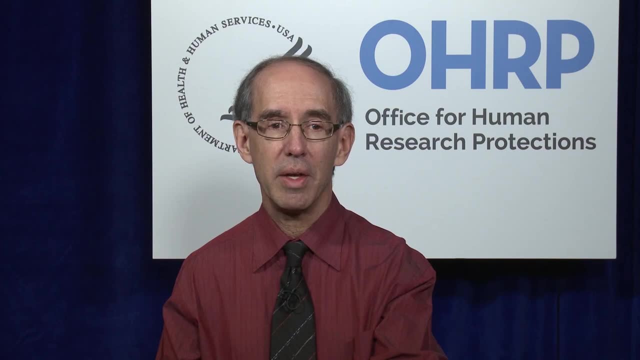 take place in the study. So the representative who has authority to consent to procedures for clinical purposes is basically allowed to consent for the person to participate in the research study. So that's what OHRP currently allows to take place. Now it happens to be the case that in some states 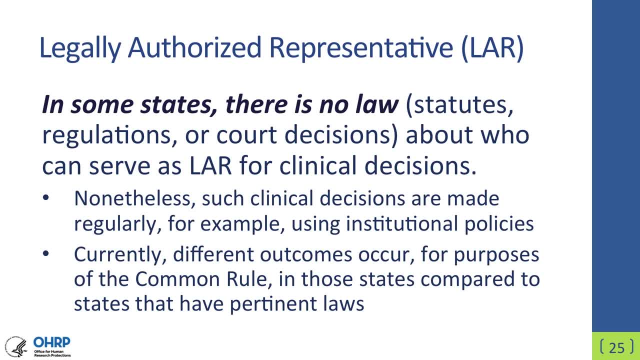 there is no such law, There is no statute, regulation or court decision about who can serve as such a representative for clinical decisions. Now, in spite of that, actually what happens in those states is probably not all that different than what happens in the states that have. 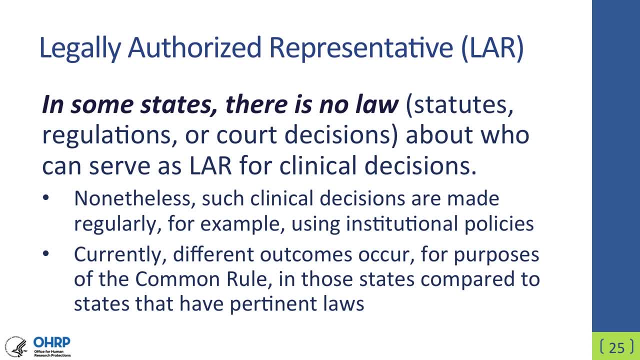 laws, because clinical decisions are made thousands of times a day, where representatives make decisions on behalf of somebody who isn't able to make those decisions, And the way this takes place is using certain types of institutional policies that are basically accepted in those states and allowed for purposes. 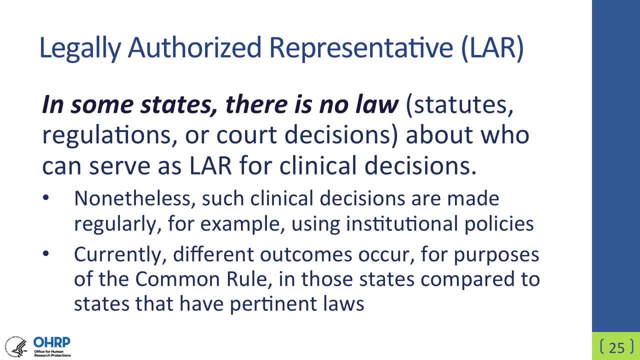 of making those decisions. So what happens now in terms of the common rule, is that in those states there's a different outcome, in that there'd be no way, or no Simple way, short of obtaining a legal guardianship. there's no simple way to allow these representatives. 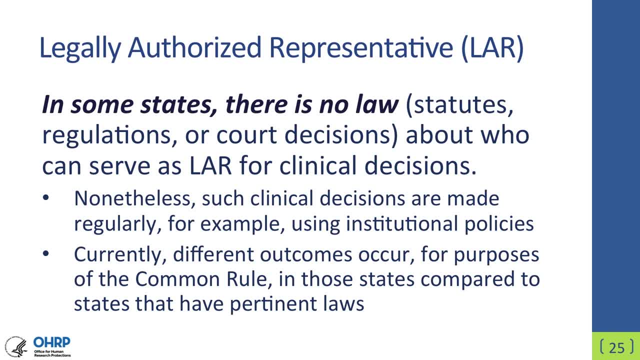 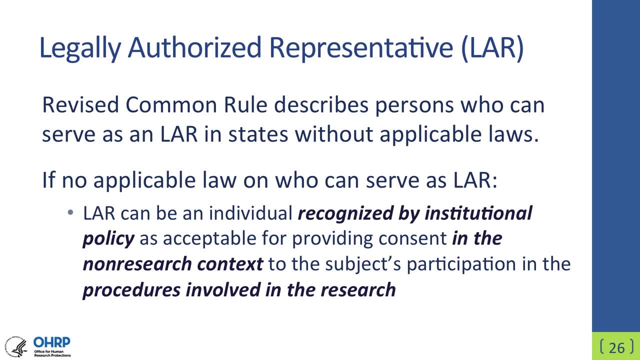 to give consent for the person who can't give consent on their own. So the revisions to the common rule try to make the outcomes more similar in the states that have the laws compared to those without the laws, because basically the same thing is happening in both sets of states. 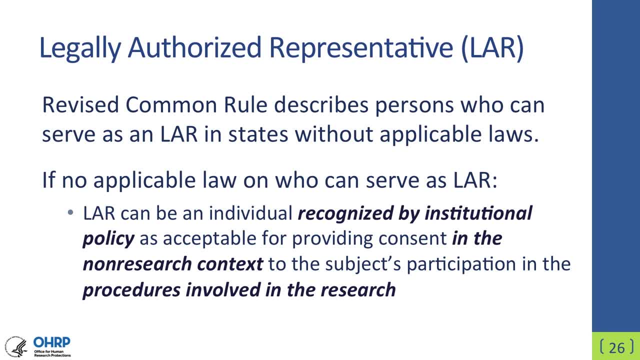 There are clinical decisions made, There's a law that allows for the use of a representative all the time by using effectively a representative. So the specific new change is that if there's no applicable law about who can serve as a legally authorized representative for purposes, 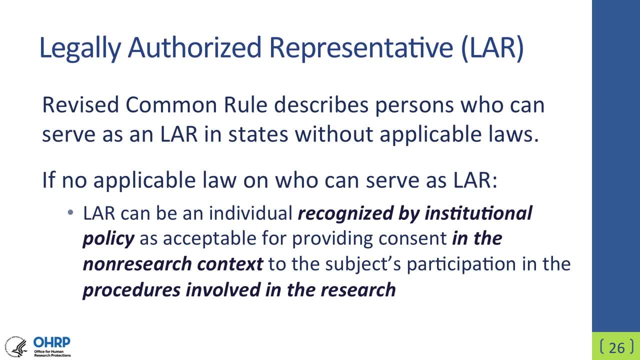 as an LAR, then in those states the LAR can be an individual recognized by institutional policy as acceptable for providing consent in the non-research context. So the LAR can be an LAR for purposes of the research under those circumstances. 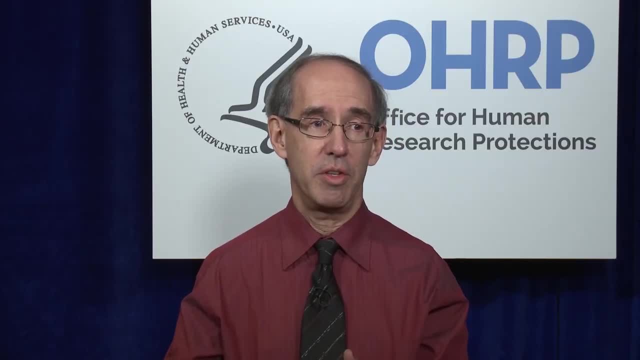 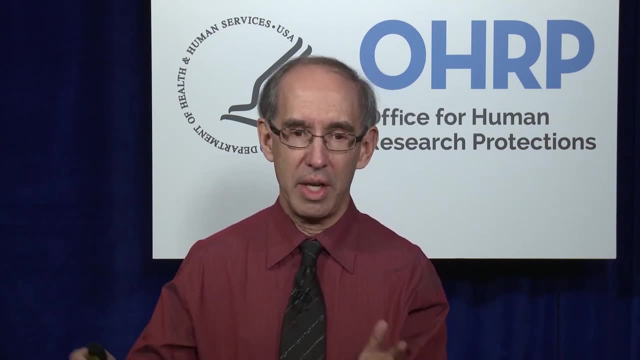 Their ability to give consent in the clinical context translates over to an ability to give consent in the research context, And again, all this is doing is making the outcome similar between the two types of states that have different legal regimes for purposes of LAR, and the LAR can be an LAR for purposes of the research. 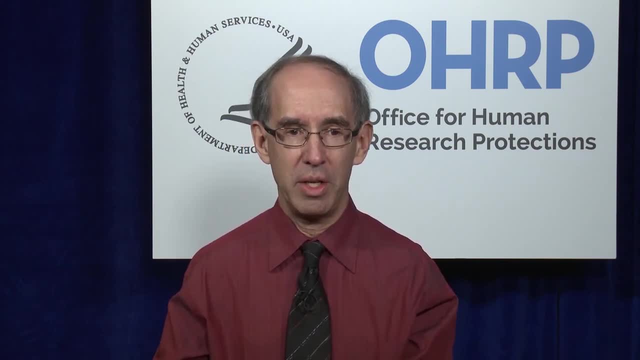 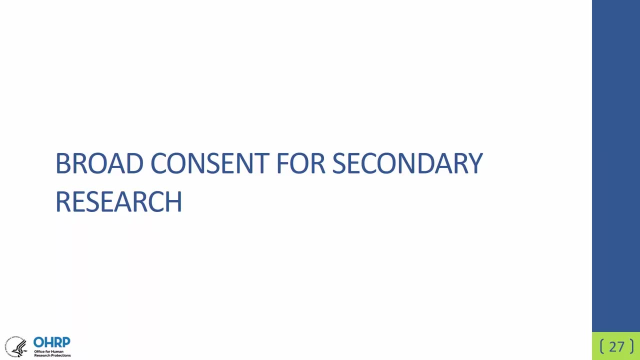 under those circumstances. So that's the way it works. So that's the way it works for purposes of LAR decision making in the clinical context. And let me finally go on to the final topic here, which is about broad consent for secondary research. 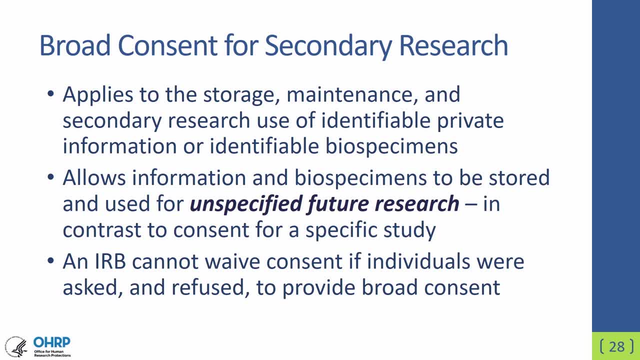 There are new rules relating to this. They're fairly complicated. They also interact with a set of rules relating to new types of exemptions, And what we're talking about here is the storage, maintenance and secondary research use of identifiable private information, identifiable biospecimens. 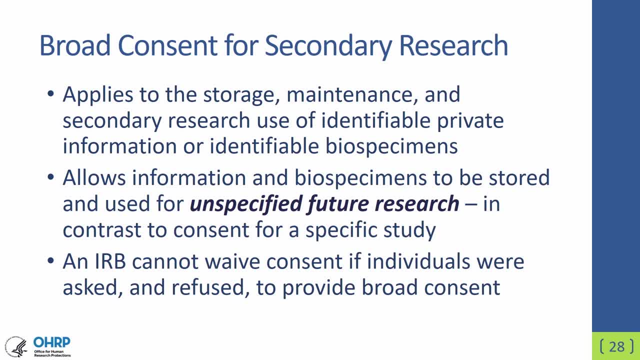 And these new broad consent rules allow this type of information and biospecimens to be stored and used for unspecified future research, In contrast to the normal scenario where you get consent for a specific study. note that if somebody is asked to provide such broad consent, 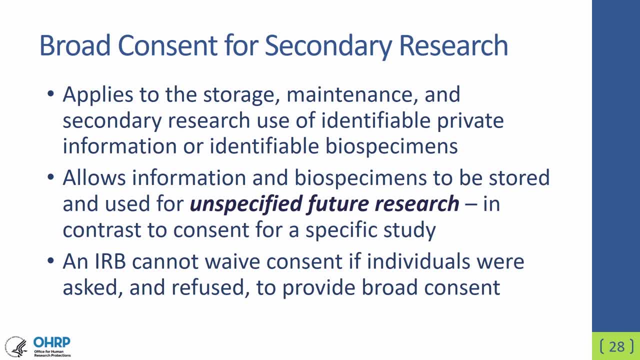 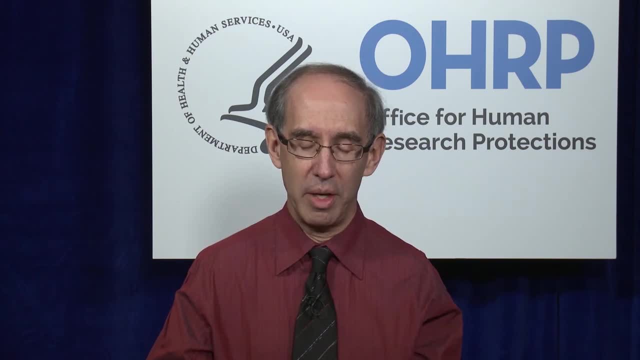 and refuse to do it, then, following that, an IRB could not- They would not- waive consent to the use of the identifiable information or biospecimens. Again, these rules are fairly complicated. There will be other webinars about them, So I encourage you to look to those for that.